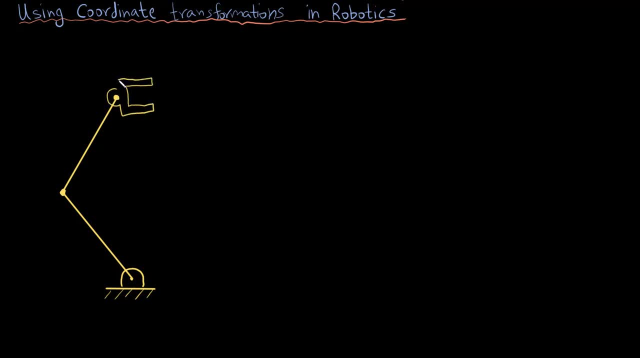 and an end effector which is a gripper, and I am marking the length of the links as L1 and L2.. Now I am drawing a fixed frame at the base of the robot, I am marking as F and I am drawing a moving frame at the end of the end effector I have drawn 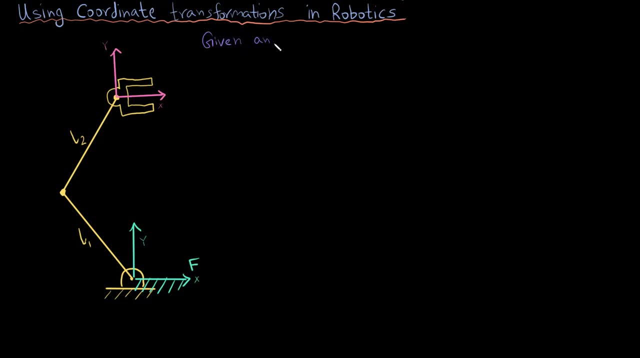 this in pink. Now the question is that I am given the position of an object with respect to the end effector frame and I now need to find the position of the same object with respect to the fixed frame or the frame which is fixed to the base of the robot. So the question is: 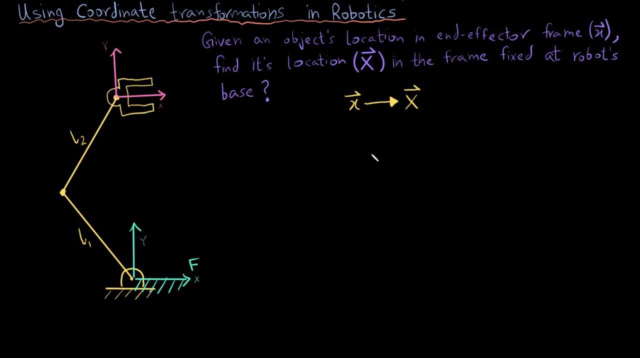 how do I go from the small x to the big X? There are a few steps that you need to follow. The first is you need to define and draw the fixed frame and the end effector frame. The second is you need to draw a frame at each of the joints, with its x-axis parallel to the next. 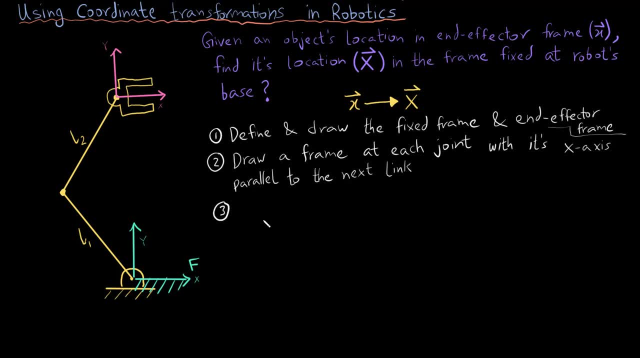 link. And the third is you need to mark out the rotation angles. There are two things that you need to consider. The first is that all the rotation angles have to be in an anti-clockwise direction, since anti-clockwise is positive, And the second? 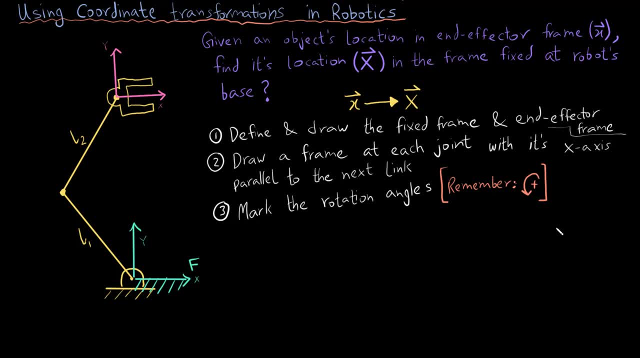 thing is that the rotation angle is going to be with respect to the previous frame. I have already drawn the fixed frame and the end effector frame, so the first step is done. Moving to the second step, I am drawing the first frame, M1.. Notice that the x-axis of M1 is: 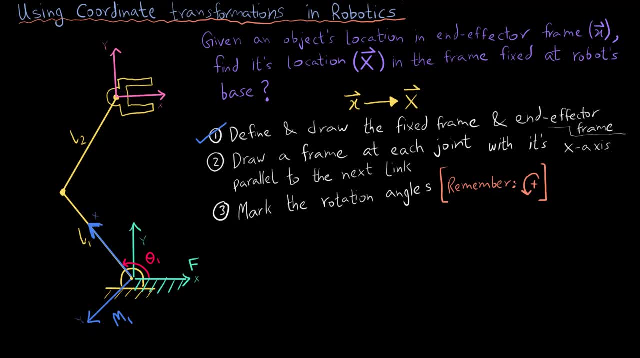 parallel to the first link and the theta one is from the x-axis of the fixed frame to the x-axis of the M1 frame. Then I make the second frame, M2.. Notice that the x-axis is parallel to the next link, A2, and the angle is between the x-axis of M1 and the x-axis of M2, which is 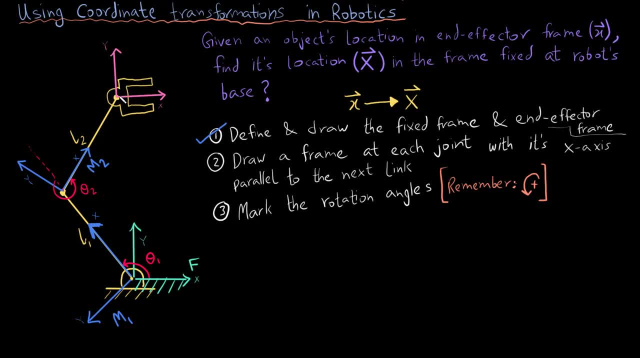 marked as theta 2.. And the theta three is between the x-axis of M1 and the x-axis of M2.. the x-axis of m2 and x-axis of m3 in an anticlockwise direction. with this done, now I can write the relationship, that is the equation of the big X, with respect. 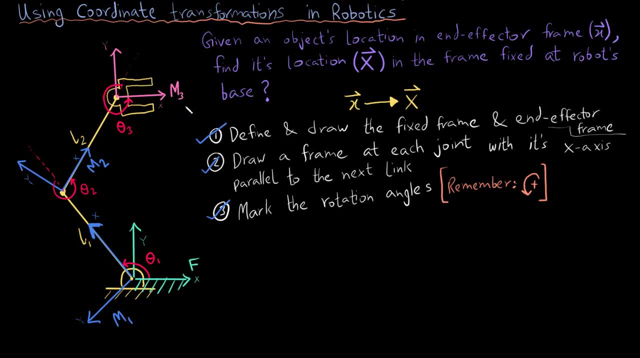 to the small X just by observing this figure. however, that does require a bit of practice and expertise, so if you are new to this, it would be better if you follow a step-by-step process. so the step-by-step process is that you write the relationship between one frame with respect to its previous frame and then 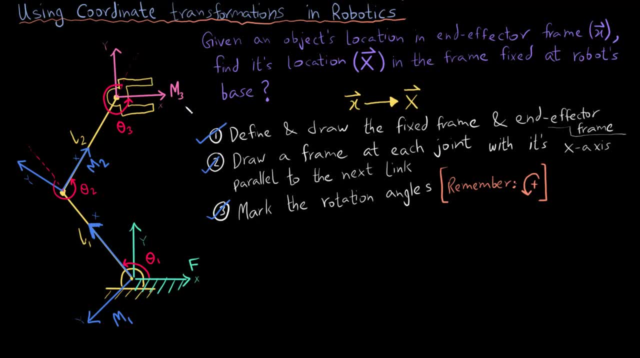 with that frame with respect to its previous frame, and so forth. I am NOT going to bore you with all the mathematics, so I'm just going to fast forward with this. if you find this difficult, I would encourage you to watch the last few videos in this video series, in which I basically drive how to 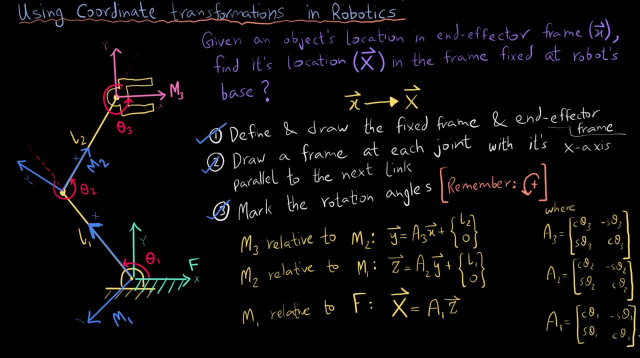 get there to this point. I just want to bring your focus to this last equation. notice that it is for the frame m1 with respect to the fixed frame F, since the origins are coincident, so there is no translation involved. it is a case of pure rotation. 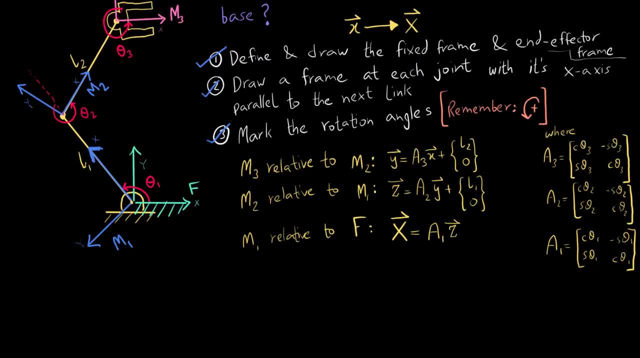 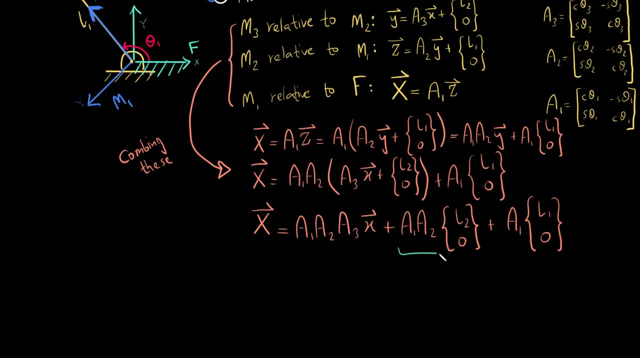 and hence there is no displacement. vector D: moving forward and putting the equations into one another and fast forwarding everything, I get to this equation. there are two terms in this equation. the equation gives me the displacement terms and the first term gives me the rotation term. we're even times A2, times A3 is the rotation matrix, and once I 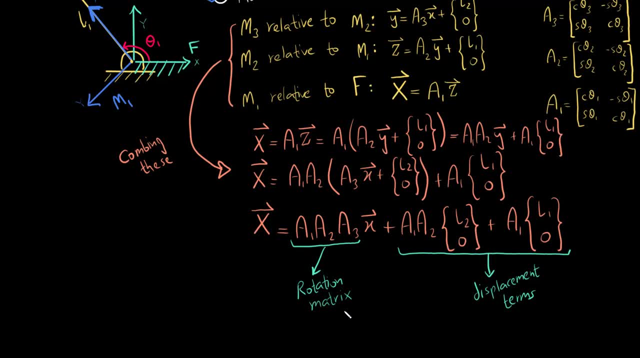 multiply A1 times A2 times A3, I get a 2 by 2 matrix which has cosine of Theta 1 plus Theta 2 plus Theta 3, sine of Theta 1 plus Theta 2, 2 plus Theta 3 minus sine of Theta 1 plus Theta 2 plus Theta 3, and cosine of theta 1, theta 2 and theta 3. 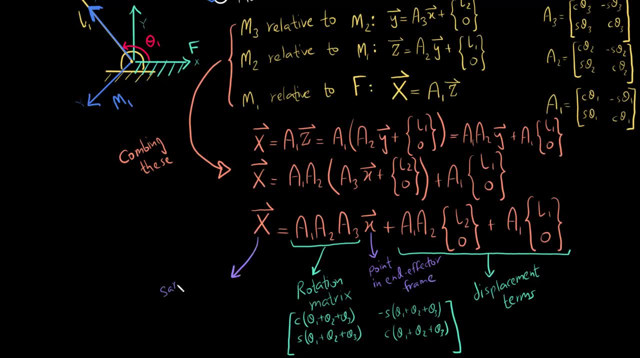 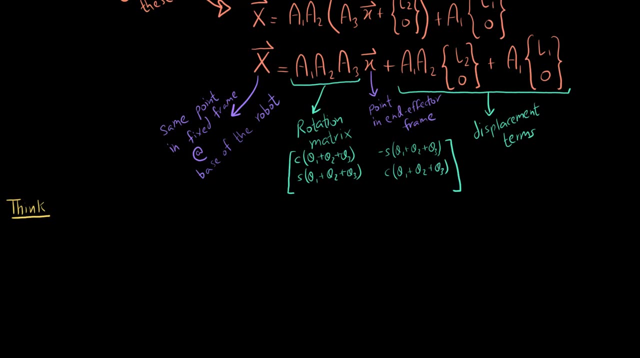 X is the point which is expressed in the identifactor frame and the big X is the same point which is expressed in the fixed frame, the frame which is fixed at the base of the robot. now I'm going to put forward a question. I would want you to put your thinking. 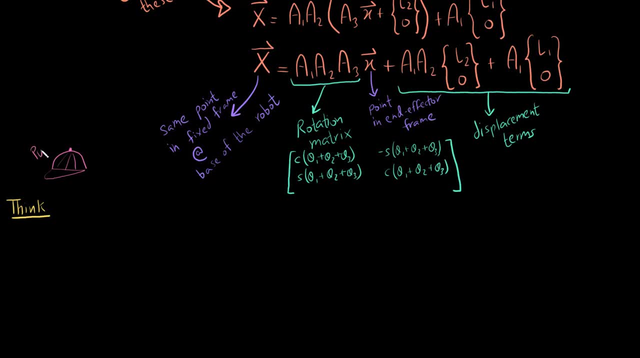 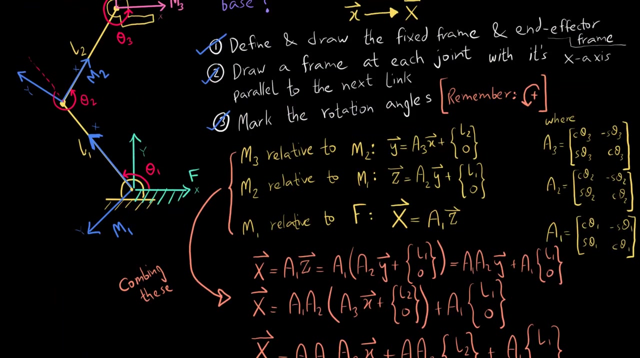 cap on and think through it. you might have to pause the video to think hard on this one. so the question is: how do I find the location of the end effector in the fixed frame, given the robot parameters? the robot parameters are the lengths of the rings, which I marked as a 1 and a 2, and the joint angle is theta 1. 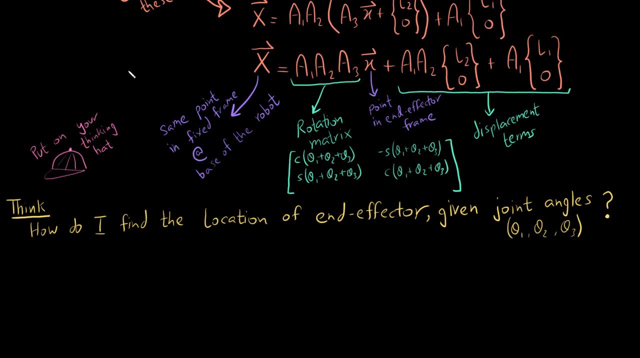 theta 2, theta 3. just giving you a small hint. you have to use this equation right here. so I encourage you to pause the video right now, think over it and see if you can figure this out. if you were able to get it, then good job. if you were in, then don't worry, let me 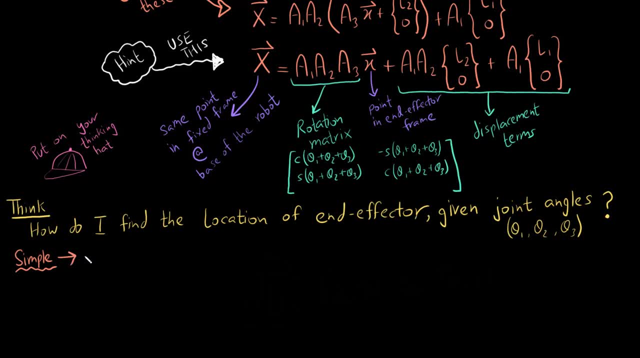 ask you a simple question and I think you would be able to answer this after that question. so the question is: what's the position of the end effector in the end effector frame? of course it's the origin. so it's 0 and X and 0 and Y. let me go up and show you. 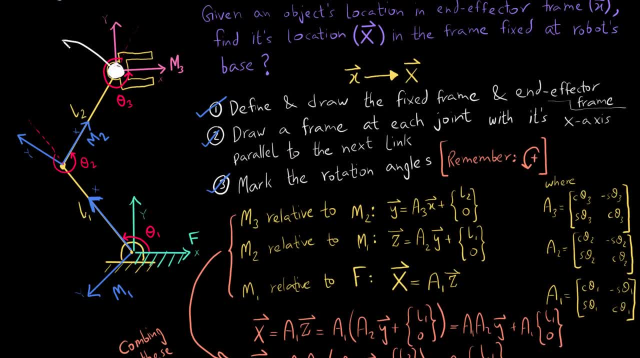 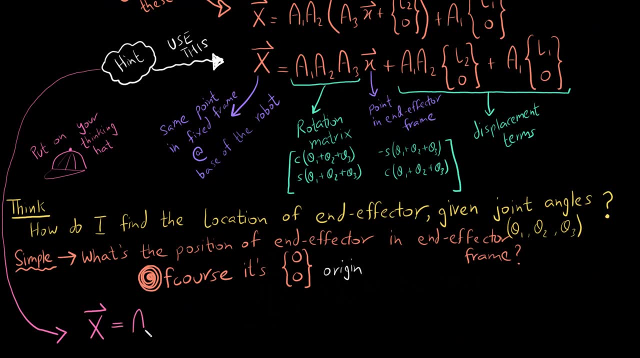 what I mean here. I am talking about this point here, which is the origin of the m3 frame. so I use this equation here, the big X equation, and in this equation I simply substitute the small X as 0 and 0. and then I just saw this equation. 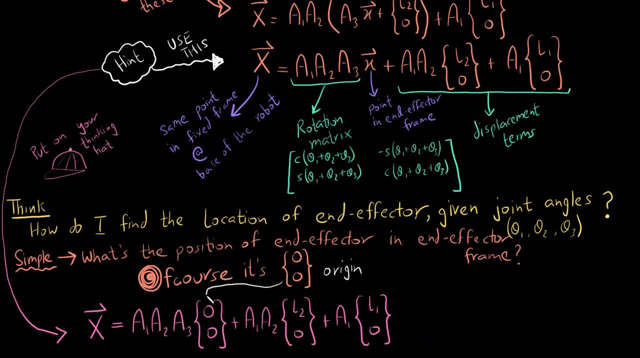 remember that I am already given the robot parameters, which are the lengths of the links a1 and a2, as well as the joint angles, theta 1, theta 2 and theta 3. so with all the unknowns known. I just saw this equation and I would get a two vector, such as 4 and 5, so the 4 would. 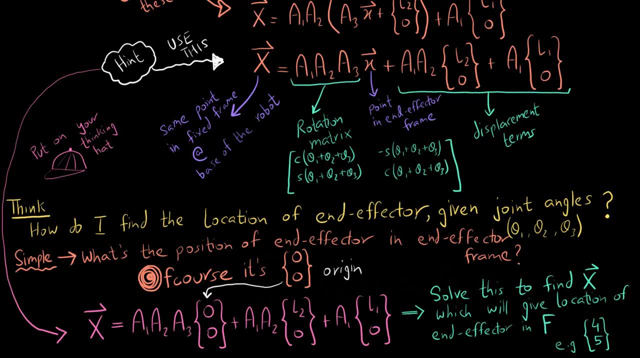 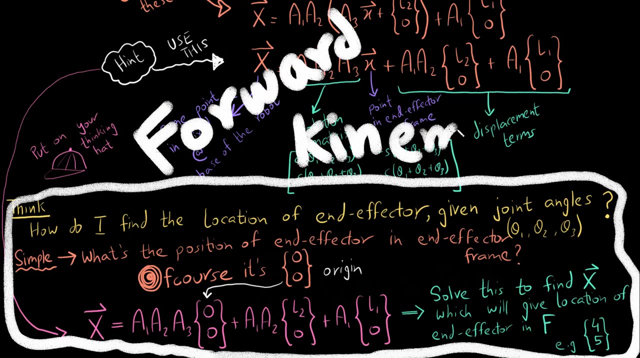 represent the X coordinate of the end effector in the fixed frame and the 5 would represent the Y coordinate of the end effector in the fixed frame. so this is what we call forward kinematics. so forward kinematics is basically given the robot parameters. I have to start from the robot parameters. 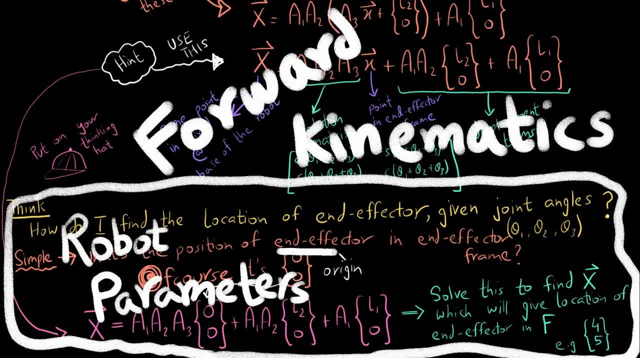 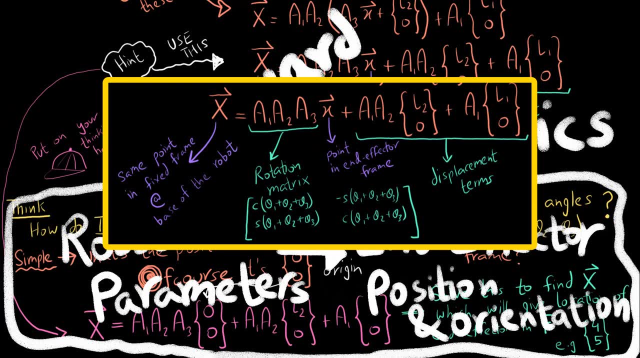 and find out the position and orientation of the end effector. the position of the end effector is the big X and the orientation is found by having a look at the rotation matrix. so in this case the rotation matrix is a1, a2, a3. if I have a look at a1, a2, a3, I can see that it has the sum of theta 1.